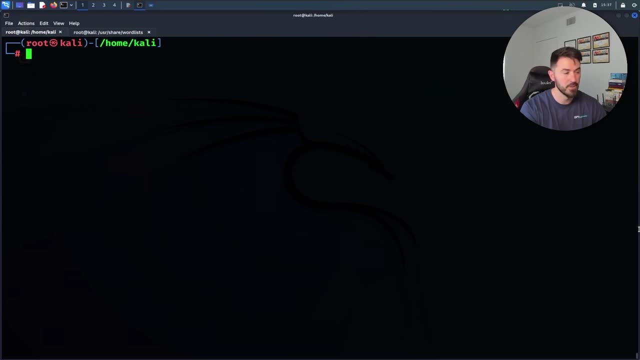 plug it in and install the drivers. So I'm not going to go over that here. So once you actually have it installed, what you can do is just run LSUSB and you can see. make sure your wireless card is there. Mine is right there. So I just wanted to put that out there before you guys say. 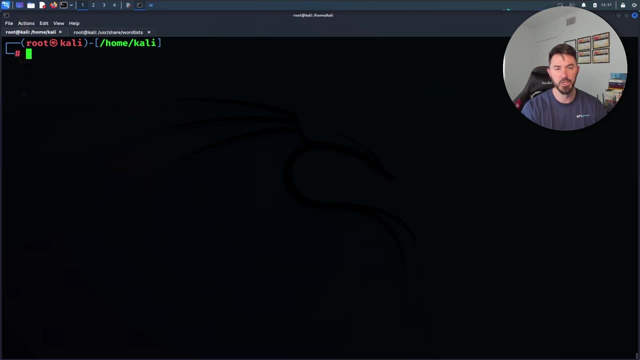 oh, it's not working. I don't get the same options as you, You know, because you need to have these tools, excuse me, you need to have these drivers and the right access, the right access points and the right cards in order to perform this. So I just wanted to put that out there before I forget. 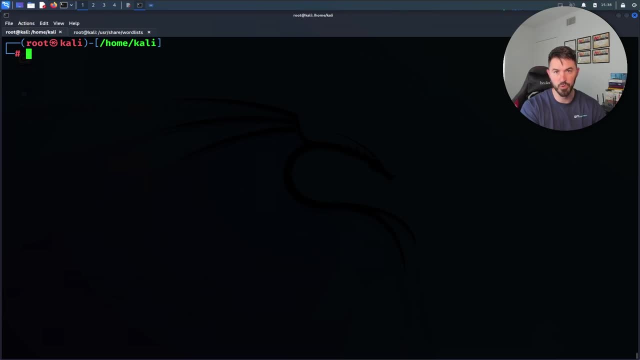 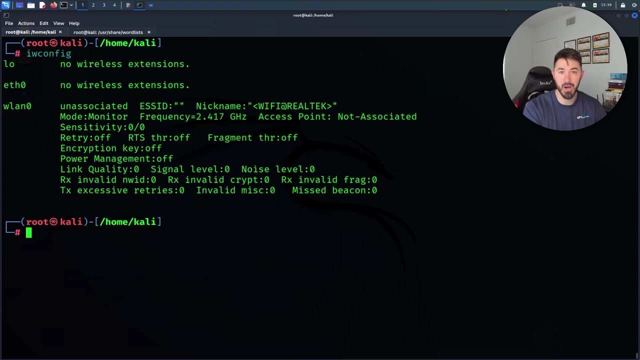 and get these crazy messages saying it's not working when I'm doing it on my laptop. But you know you need an external card, All right. So first thing we can do is do an IW config just to make sure we have our access point, our card, in monitor mode. So what is monitor mode? 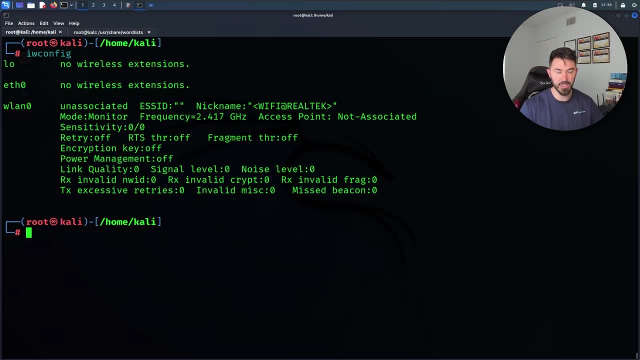 So you have two modes, right. You have manage mode so you can get onto the internet, You can. you know all the default. by default, everything's in manage mode, right? So when you put it in monitor mode, that means you're allowed to listen for packets. You're listening, you know, you're. 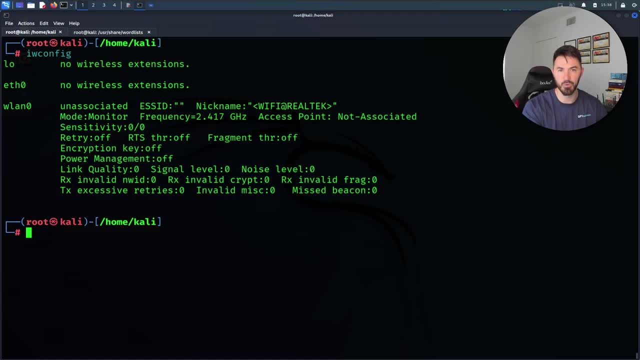 able to ingest data, You're able to listen for packets. You're able to listen for packets And, you know, sniff the networks. I guess you can say right. So if it's in manage mode- excuse me, monitor mode- you're good. If it's in manage mode, what you can do is run a command. 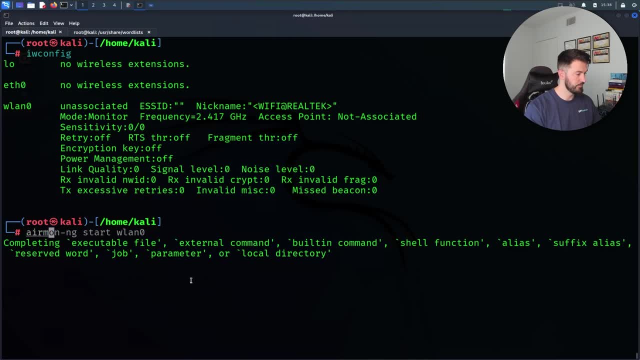 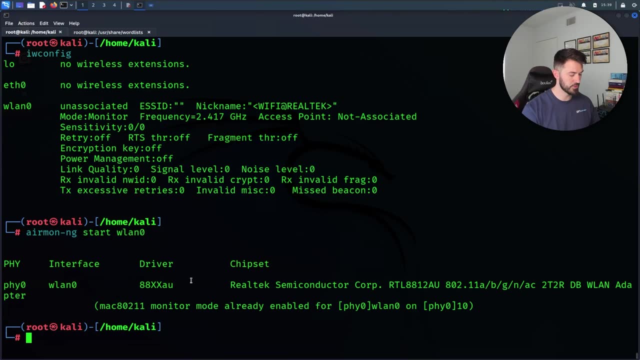 air, air mon ng start and then whatever, whatever interface you're on. So I'm on WLAN zero, So you just do that, And then you can just run it again and you should be in monitor mode. And those are the you know. 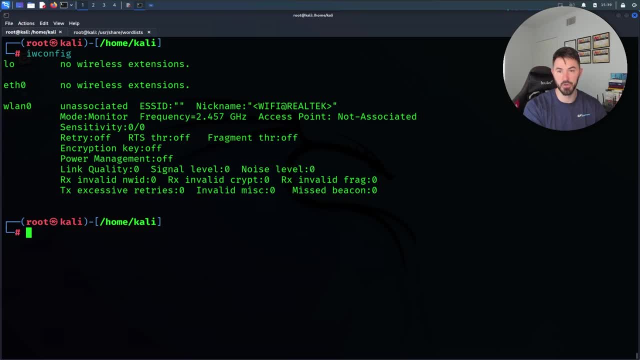 a few preliminary steps you should take to make sure you're good to go. So now what we need to do is stop capturing packets And we can use a tool called arrow dump ng. This is the old you know at crack ng suite. So you know, just learn how to use this if you're definitely interested in. 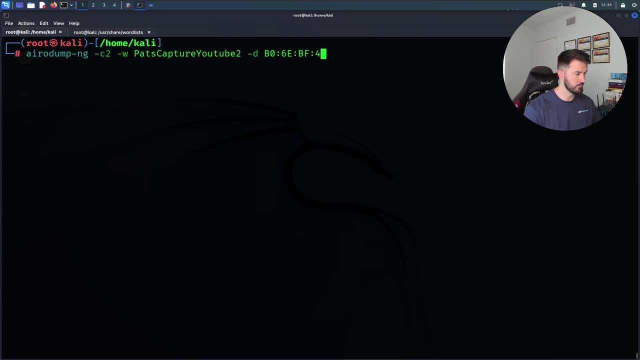 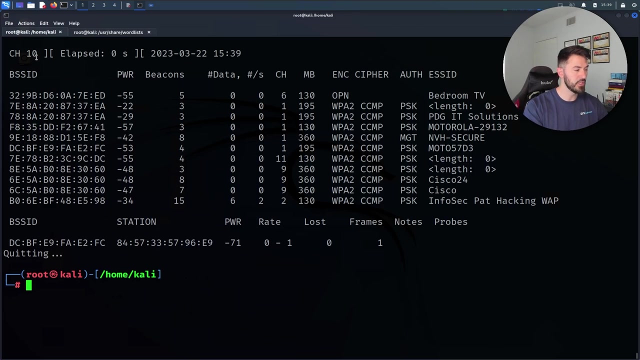 wireless hacking. So you can do arrow dump ng, not that. So arrow dump ng wireless of WLAN zero. So now I want to go ahead and just control C. I want to stop that. So up here, what it's doing up here is: 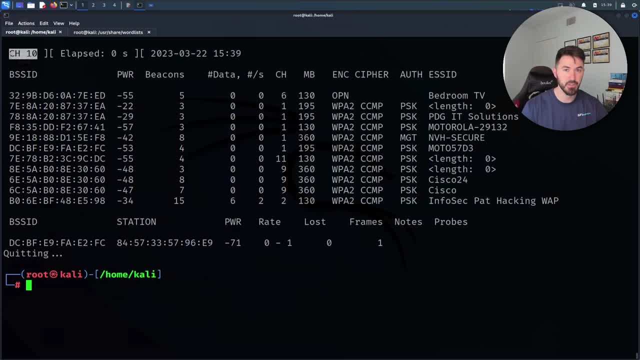 which is known as channel hopping. It's hopping the channels, jumping from one channel to the next channel, to the next channel. So you know, we can see here in this row, right here with the channel 6,, 1,, 11,, 9,, 2,, etc. So you probably guessed it right. The network that I'm going to be targeting is my own. 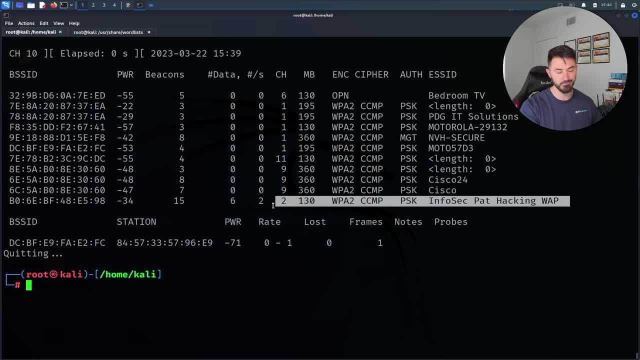 which is InfoSecPack. At that happened. it stands for a Wireless Access Point. Now, I almost said something else by accident, But yeah, so this is the information that we have gathered, So let's go ahead. I'm just going to copy this for now. 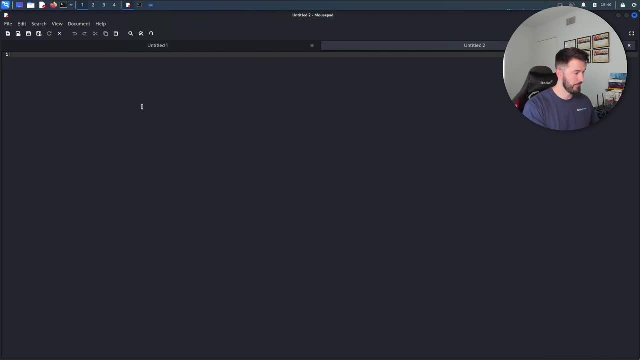 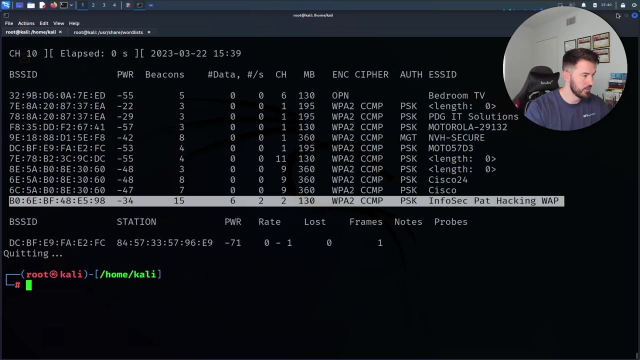 And let me just go ahead and throw it in here, And I can make this larger, just for Leda, Right? So we'll have this for Leda, Okay. So now, once we have this information, what we can do is take it a step further, and we can. 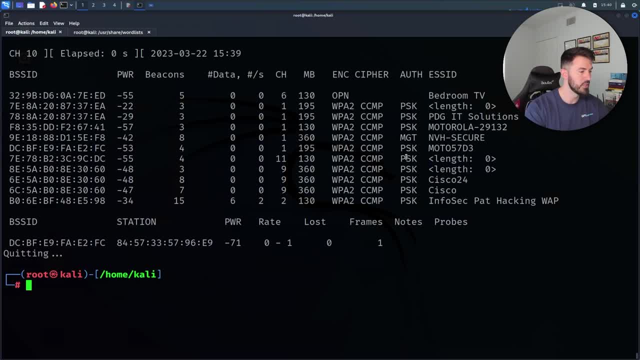 actually target just our network, right. So this is our network right here. We just got it right. So let's go ahead and just run arrow dump ng, again arrow dump ng, And then what I want to do is dash c channel, I want to channel two, because this is the channel I'm on right- And then the. 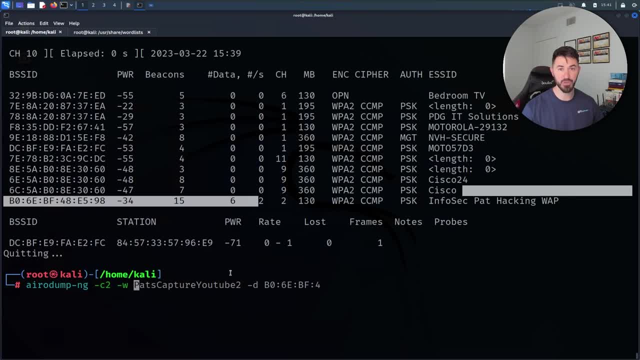 output file that I want to put it out to. I can put it to capture capture path. I don't know capture path. Okay, So now we can do a dash d And what I'm going to do is associate my access. 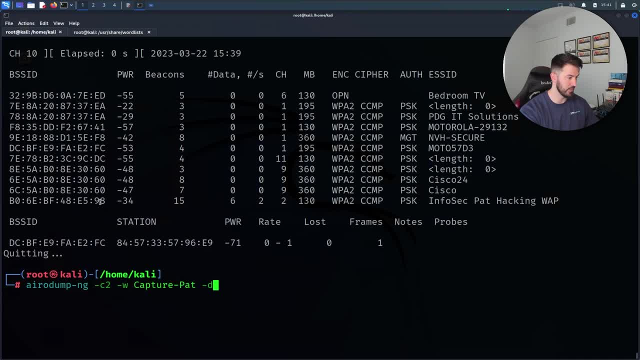 point, right, If that makes any sense. So what I'm going to do is copy this. Let me go ahead and hit space and go ahead and paste this here, And then we have to do WLAN zero, right, Because that's what I'm doing. So now this is only going. 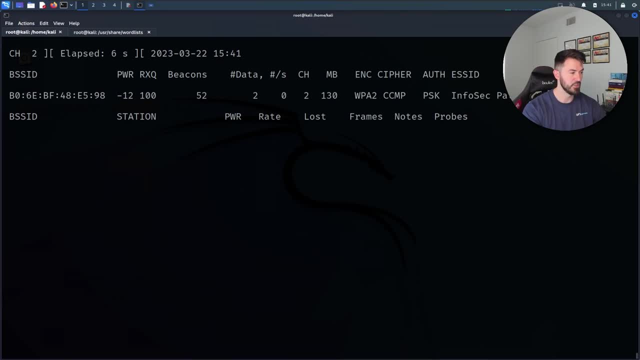 to target my network specifically. It's not going to, you know, it's not going to jump around to the other networks or anything like that, So we don't have any access, any stations connected. I do have a station. I probably got disconnected. Oh there, it is All right, So I do have my iPhone. 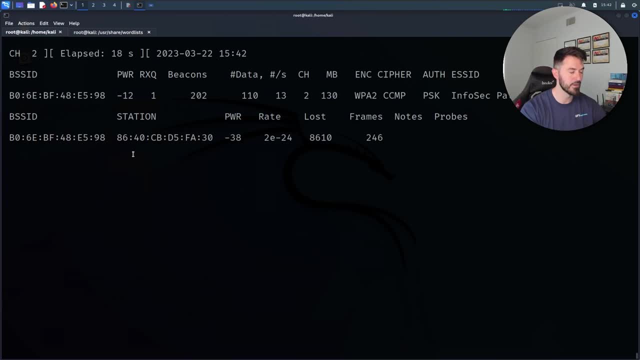 connected. So this is my iPhone right here. So the next thing we need to do is we need to deauthenticate right. So we need to deauthenticate our network. So we need to deauthenticate our. we can do a deauthentication attack in order to get the four-way handshake right. So now this is. 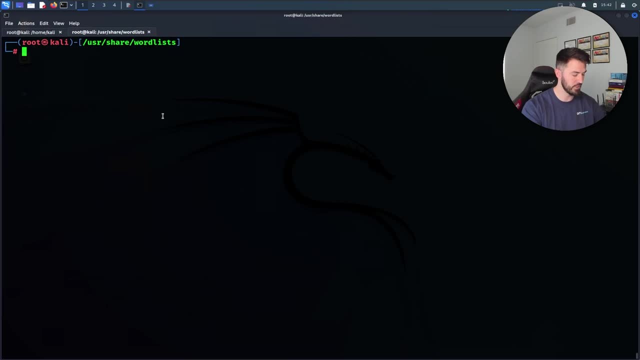 just just chilling out here. So what we can do is come over here and what we can do is air play NG. I have it here, Okay. So deauthentication zero for unlimited times. dash a, we have our access point right And then and then the client right. So this is my client, that I'm 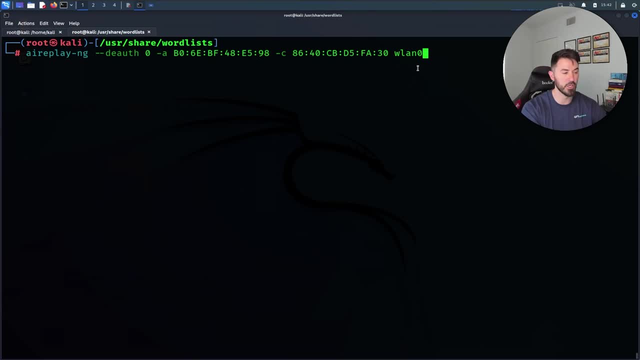 going to be removing, which is my iPhone, And then I'm going to be using my WLAN zero as my interface. So now this is going to go deauthenticate. This obviously can take some time. Let's go back here. This can take some time, depending on how far your access point is from you, How many, how many. 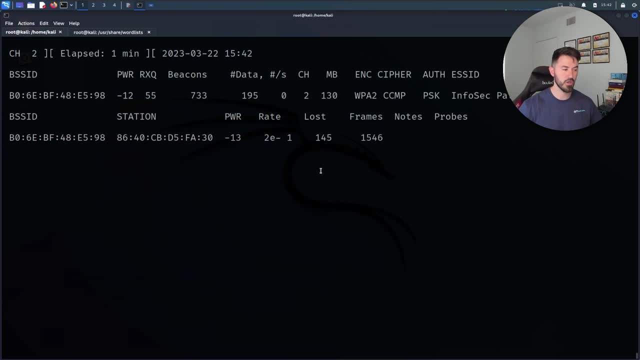 clients are connected. So obviously this is the process. I want to make this a little quicker. So what I want to do is I'm going to actually go on my iPhone, disable my wireless, enable wireless, So then it can intercept that traffic. All right, So let me do that really. 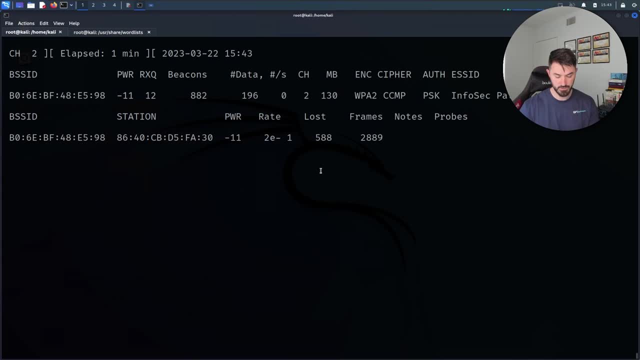 quick, Let me go ahead and turn this off, turn this back on, associate myself, and then we should get it shortly Once. uh, let's give this a second. Let me go ahead and shut this off again, Turn it on And uh, let's uh give this a moment. 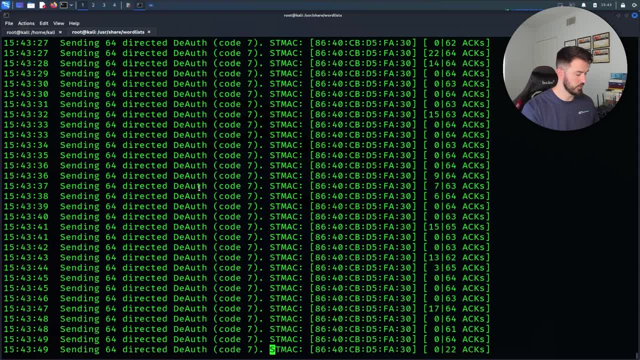 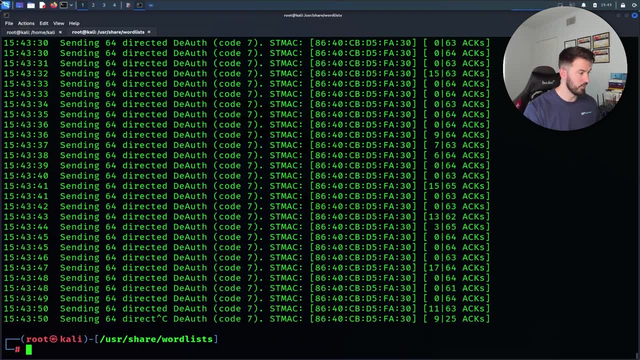 All right, So what I'm going to do, it's probably because this is doing the deauth, So I want to go ahead and cancel this Now. oops, I don't want that one, This one, Now what we could probably. 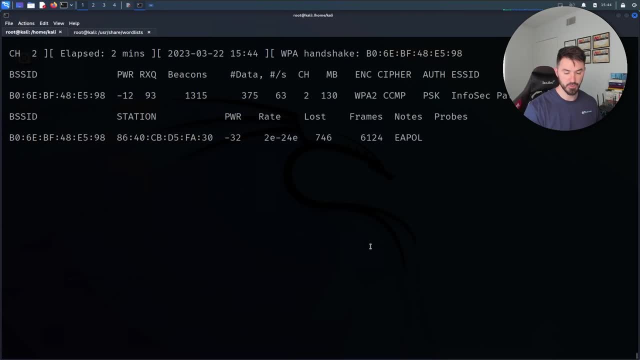 do is come back here and here we go. Okay, So that's pretty much the process. So we just, you know we spent a lot of time on this, So I'm going to go ahead and cancel this. We, uh, we cheated a little bit, right, So we can just go ahead and control C. this We already got. 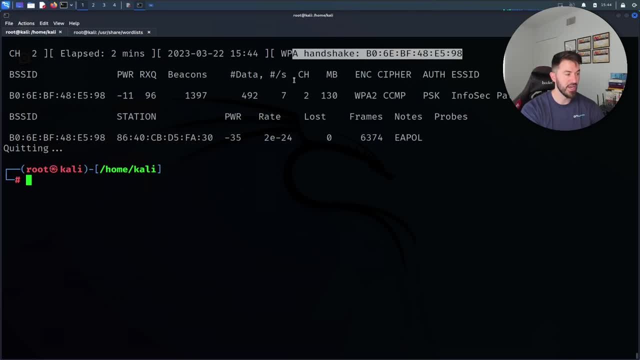 the, the four-way handshake up here. So now if we do an LS here, we have a few captures. So we have the most important thing- is the PCAP file right? So this PCAP file is super important to us because in order to do a dictionary attack or offline brute force attack or whatever kind of attack, 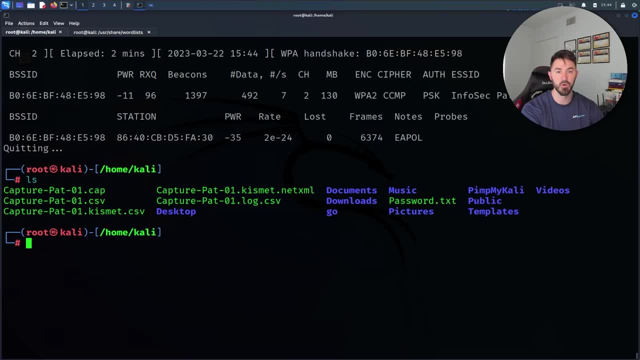 that we want to do, we need this File in order to do so. right? So what we can do is, if you want to get a little nerdy for a second, we can open this up with Wireshark and look at it. So let's do that, Let's do Wireshark. 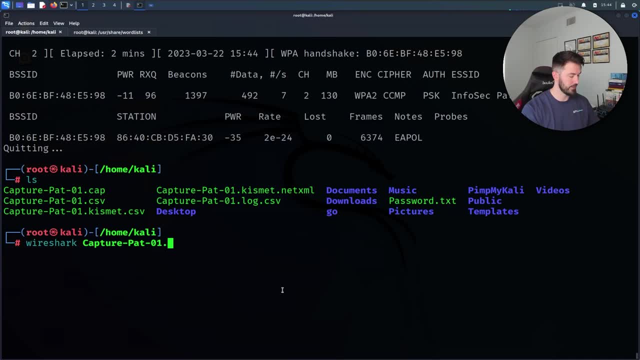 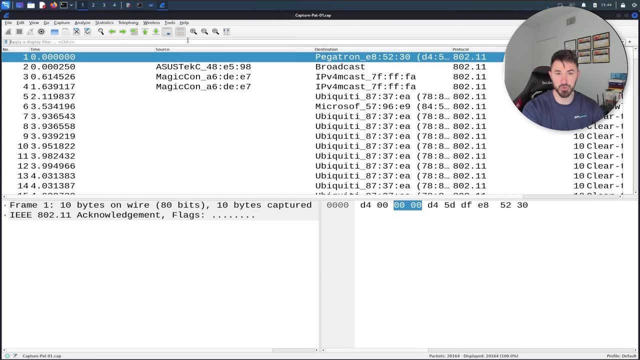 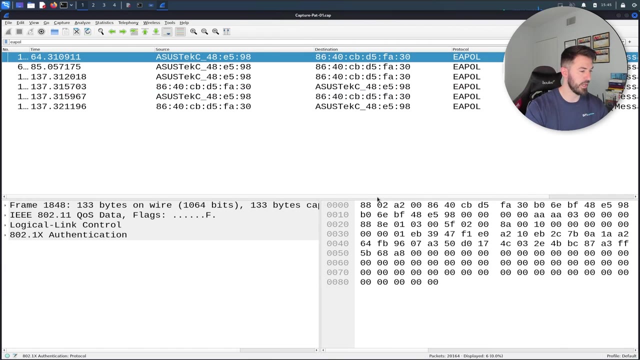 and then capture. Okay. So let's pop open this bad boy in Wireshark So we can look at the protocol that it's running on, which is EAPOL, So EAPOL. we can look at the four-way handshake here. 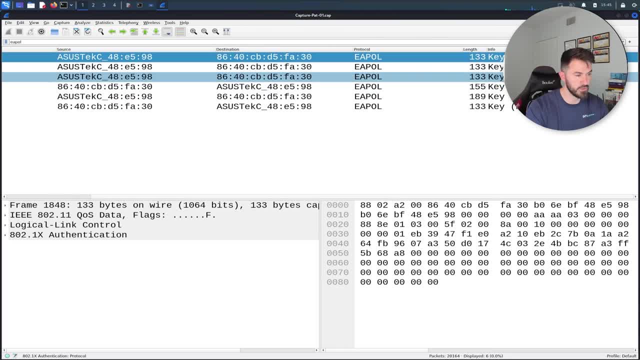 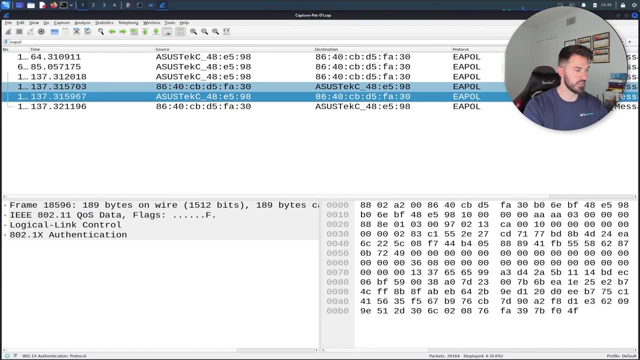 And we can look over. we can see message one, two, three, four, And these are all the messages that we, that we see here. You, you know you can do this. You can get a little nerdy. This is my. 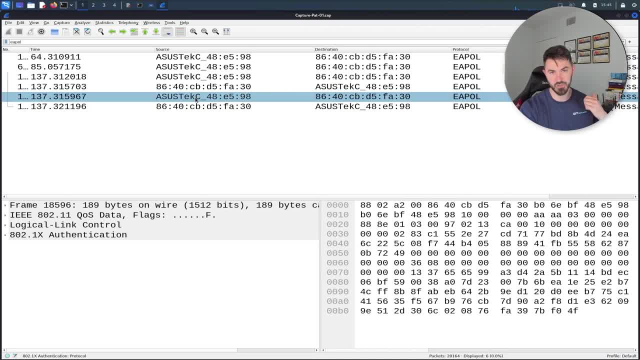 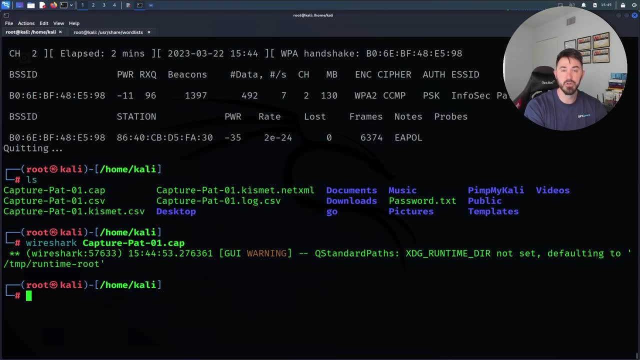 this is my phone, This is the. the ASUS is my, actually that my actual access point and all that good stuff. So you can get a little nerdy and look into here. but yeah, so that's, that's pretty much. you know how you can look into the packet level. So now what we can do. 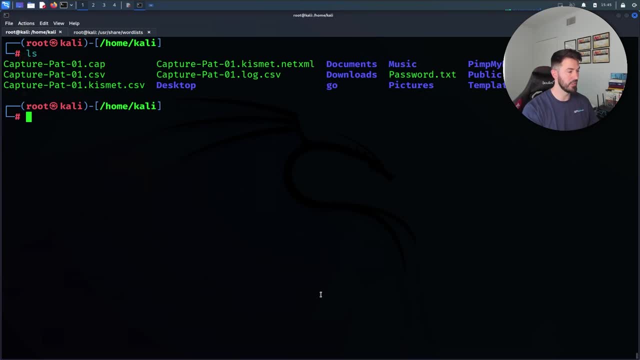 which is the most fun part. So I have. I'm going to do an LS really quick. I have this password dot TXT. So if I do a word count on password dot TXT, it's only 174 words. So it's going to be. 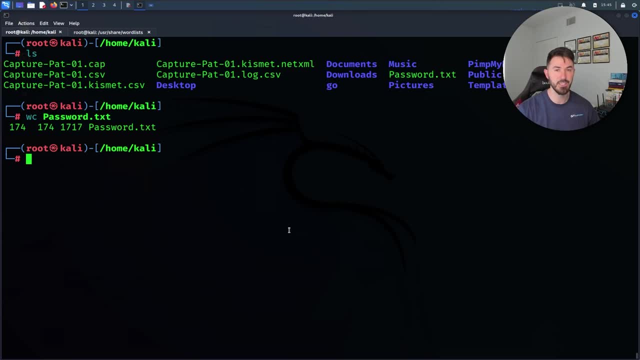 super quick, right? Maybe you're using rock, you dot TXT, Maybe you're using a sec list, Maybe you're using your own that you found on the internet wherever you you know wherever you found your word list. But what I want to do now is use aircraft. So aircraft.